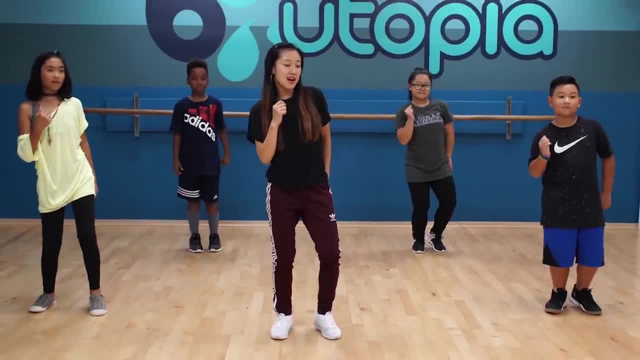 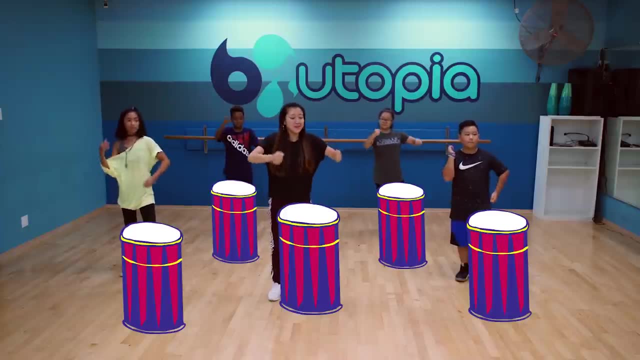 going to go one, two, three, tap, Nice, And then with your arms I'm just kind of switching like this, Like kind of like I'm drumming Like woo, drum, drum, drum. Yeah, So you're. 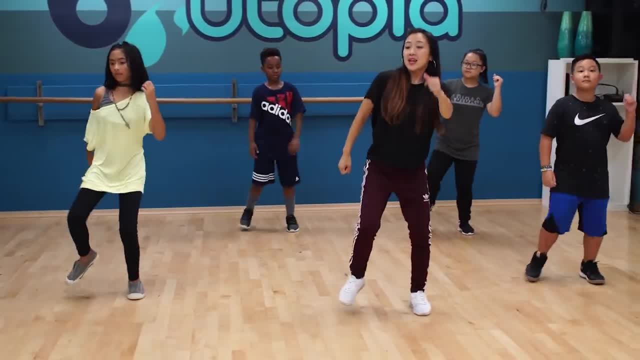 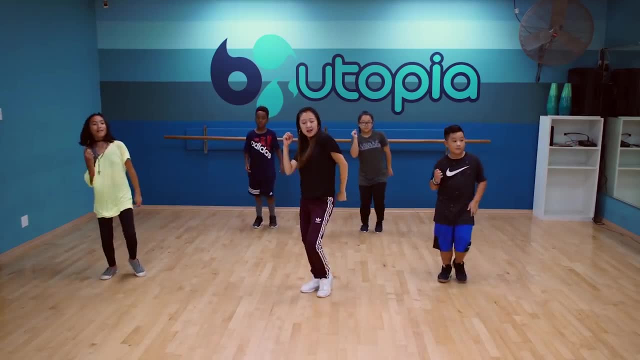 going to go. one, two, three. tap. One, two, three. Yeah, Make sure you add a little bounce. Oh, oh, oh, oh Nice, So that's called a grapevine. From here. my legs, my feet, you're just going. 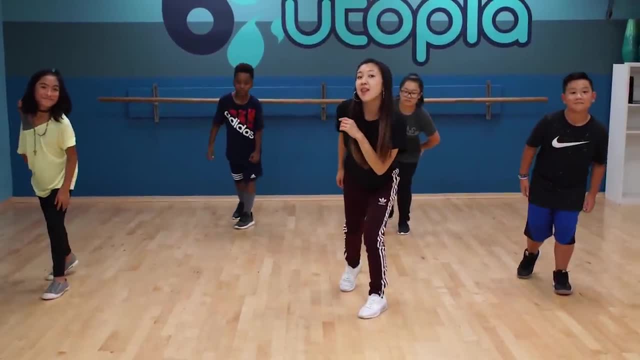 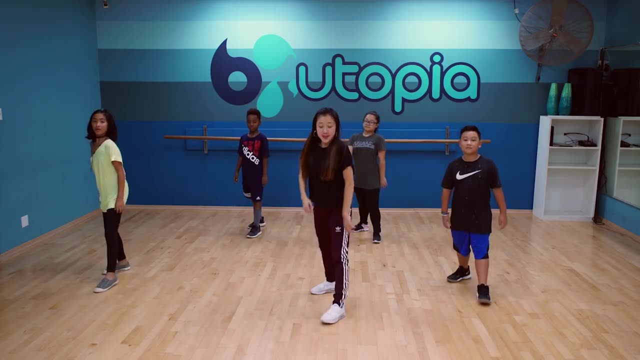 to step forward And then tap back, And then that back leg you're going to go back and tap. So it's forward, tap back and tap And make sure your weight is going also rocking back and forth. Yeah, 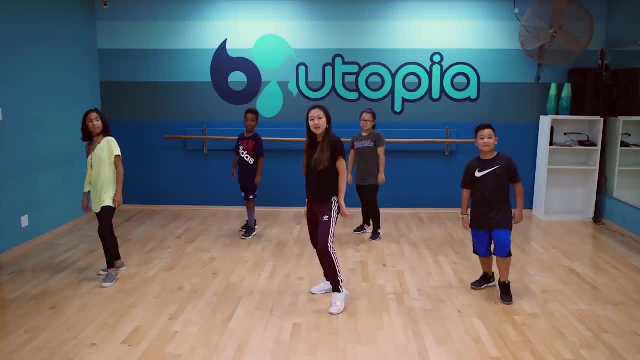 Rocking back and forth Nice, And then for our arms, we're going to pretend like we're like favorite singers. Who's your favorite singer? Who's your favorite singer? John Billion, please. Who, John Billion? Oh, I don't think I know. Oh, who's your favorite singer? My? 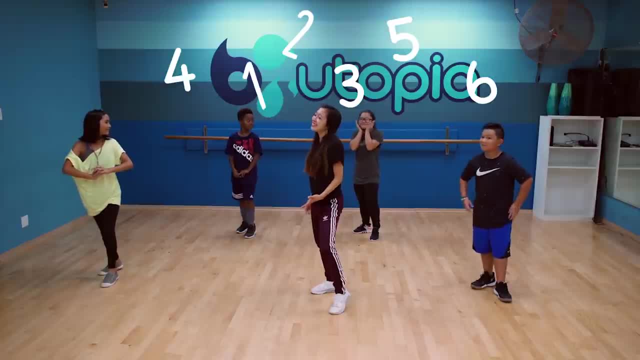 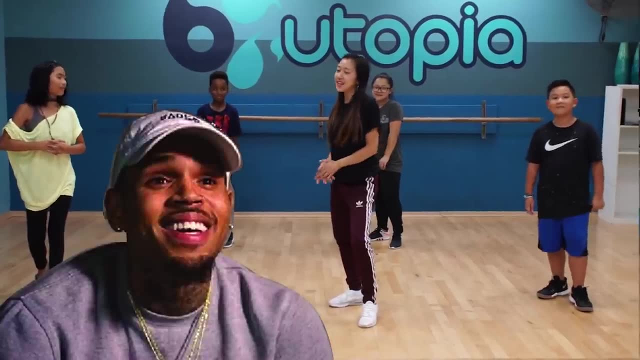 favorite singer is: I have too many, Oh too many to think of. All right. Well, let us know whenever we got. Okay, here we go. Chris Brown, Who? Chris Brown, Chris Brown, All right. Shout out: Chris Brown, All right. So we're going to bring out the microphone. 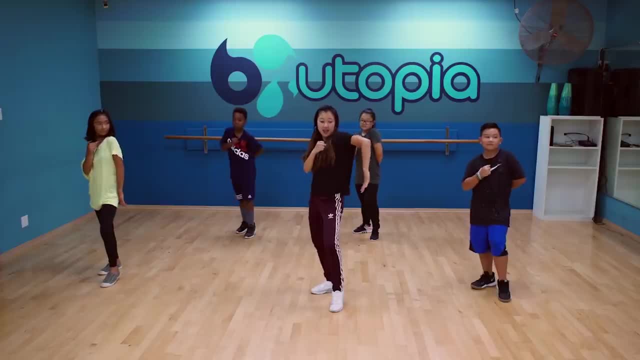 And then you're also going to shake your shoulders And this hand right here is going to hide right there. You're going to shake your shoulders up and down, Yeah, And the whole time we're going to do it with our step. All right, We're going to go step and step and step, hanging. 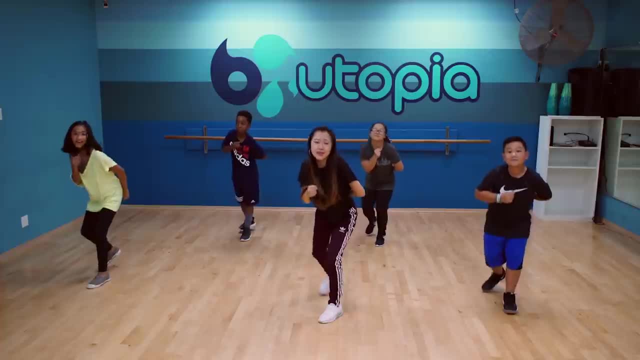 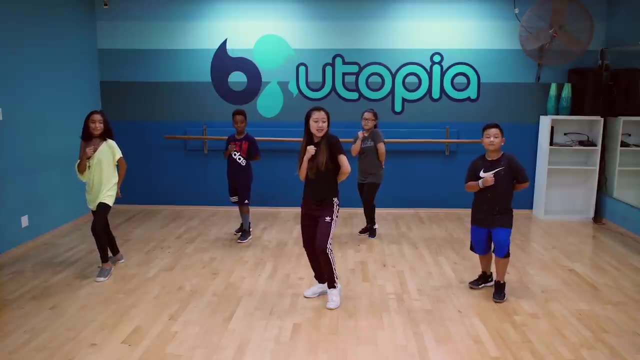 like you're sitting, Like you're Chris Brown or whoever you like. Yeah, Hey, hey and hey. And from here our feet is basically a nice little two-step. You're going to go, step, tap, step, tap, step. 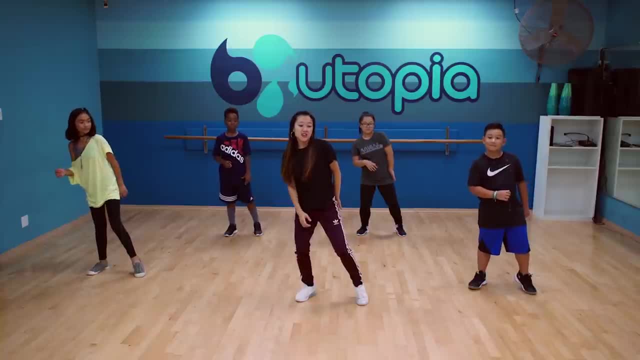 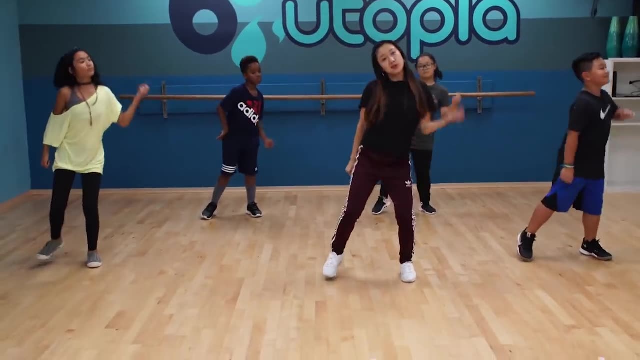 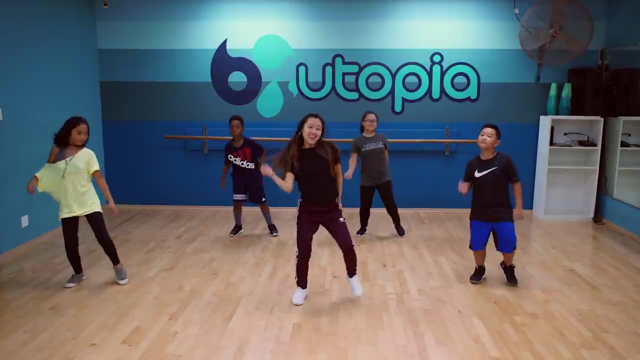 tap and step, tap, And then our arms, you're going to roll it down. your body Roll, Yeah, Side to side, And then you can go a little lower. Oh yeah, All right. And then you're going to go a little higher. Hey, hey, hey, Nice. And then from there we're going to. 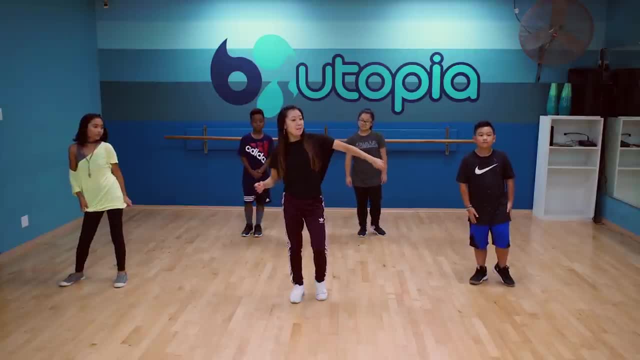 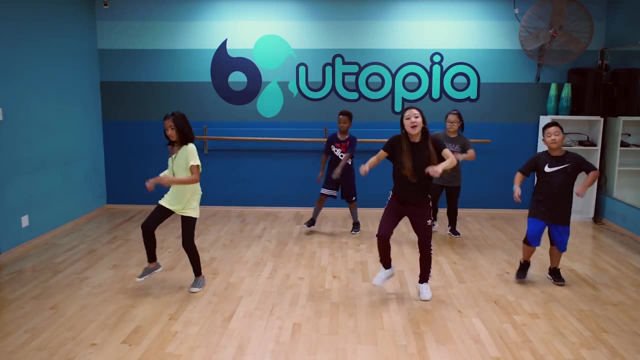 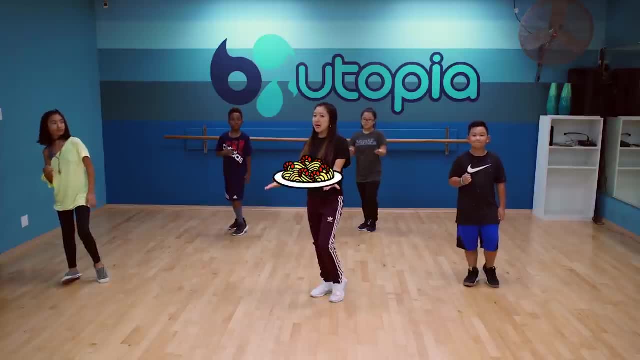 like we're serving some shrimp scampi And then we've got this big plate of pasta And you're going to just go serve it. Two, three, tap One, two, three, tap One, two, three. 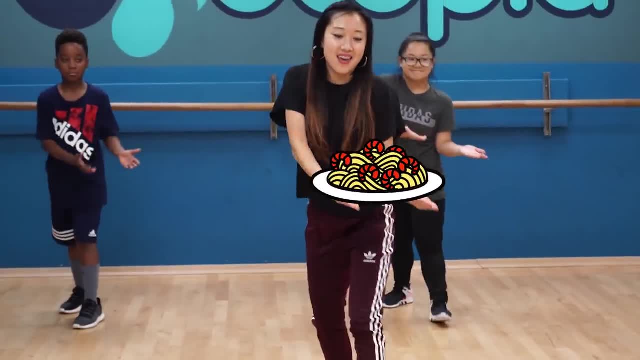 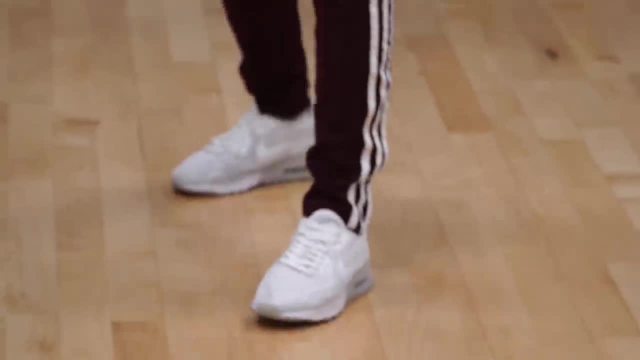 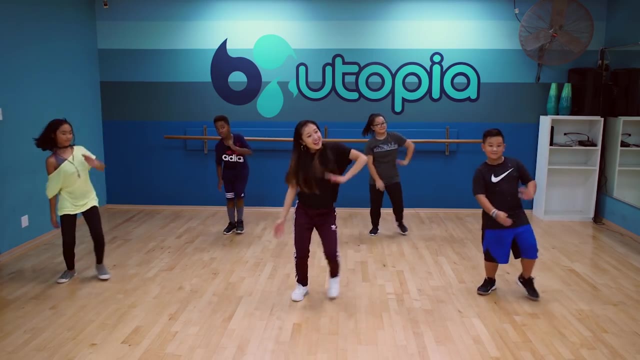 tap One, two, three tap And then you're going to serve it to your friend. Hey, Yeah, See my feet. I'm still stepping forward and back, And forward and back, And from here we're not going to roll down our body, but we're going to comb our hair. Yeah, Like 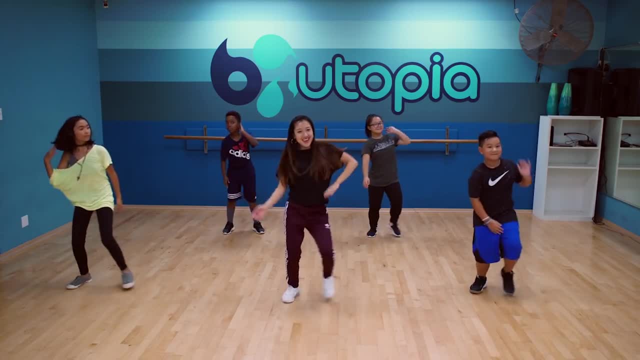 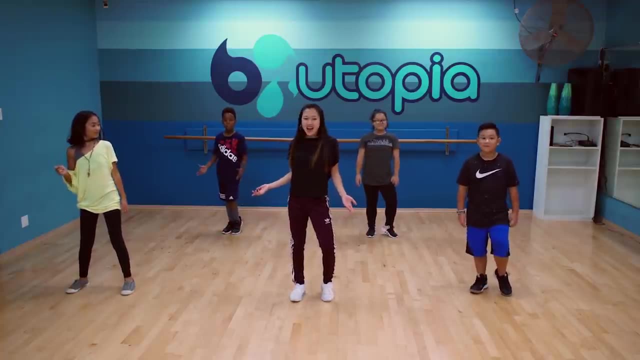 hey, it's time to get a haircut. Yeah, Hey, Woo, Nice Cool, All right, Do you guys want to hear the music? Sure, Yeah, Let's try the music. Hey, hey, hey, There is a condo in Manhattan. 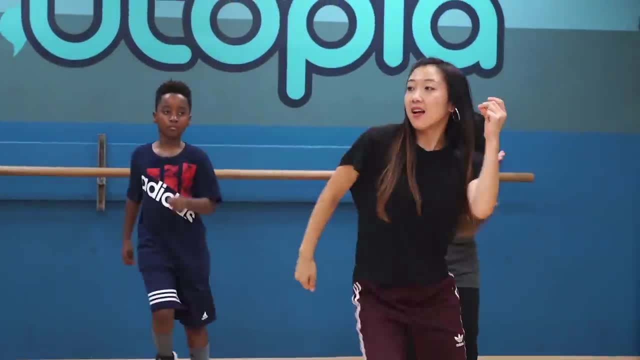 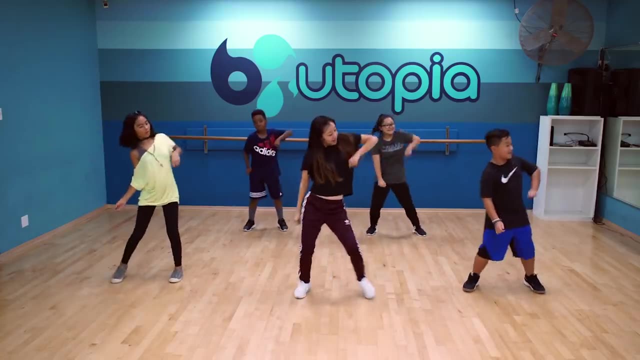 Hey there, hey, what's up? You know fans invited, So go and get to dancing. Hey, sing it with a friend. Sing it, sing it for me. Come on down and dance it with a friend, Dance it, dance it with me. I have a bitch house in Miami. 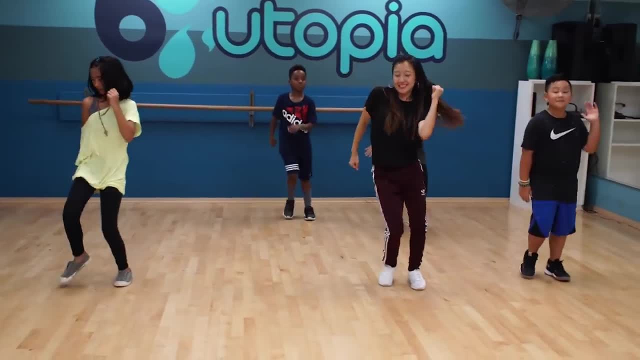 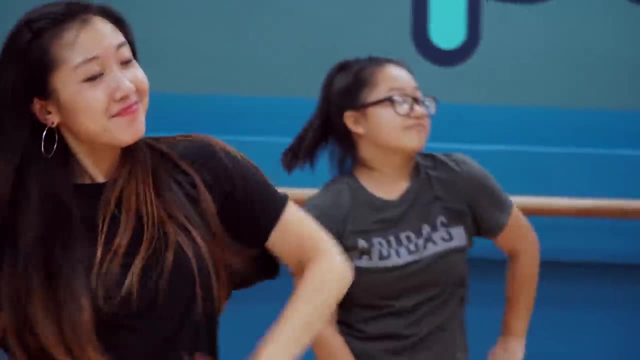 Hang out in my jammies Lobster tail for dinner, Then reserve that scampi. You got it if you want it. Got it if you want it. Said you got it if you want it. Take my wallet if you want it. Yeah, awesome, Good job you guys. 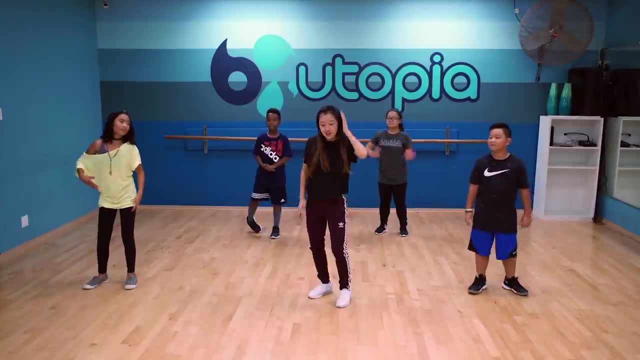 Alright, let's finish it. So we just, you know, comb our hair, comb our hair and we're about to, like, go to the beach. Yeah, we're about to go to the beach Drive. in my catalog, I wish I had one, but I don't. 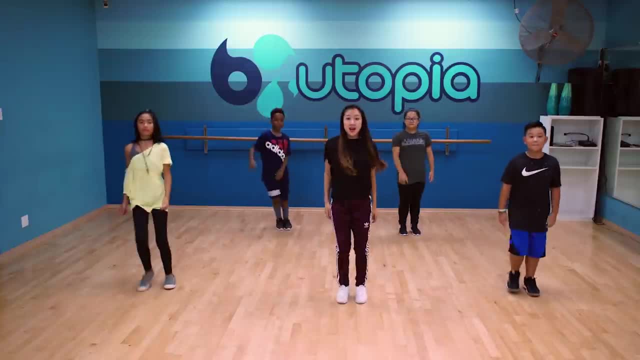 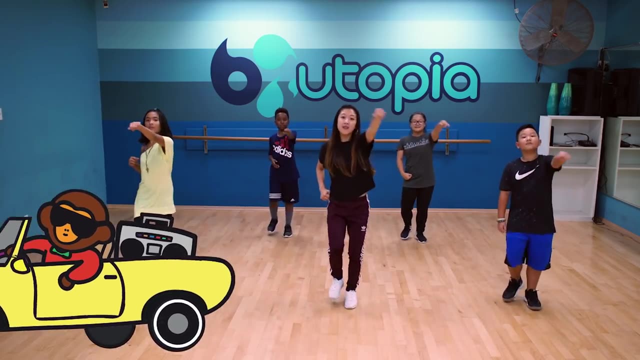 So we're gonna jump, Jump with this foot. You're gonna go jump in the catalog, You got that wheel there. You're gonna go drive, drive, drive. Hey, Nice, From here our feet. you're just gonna go, just follow my feet. 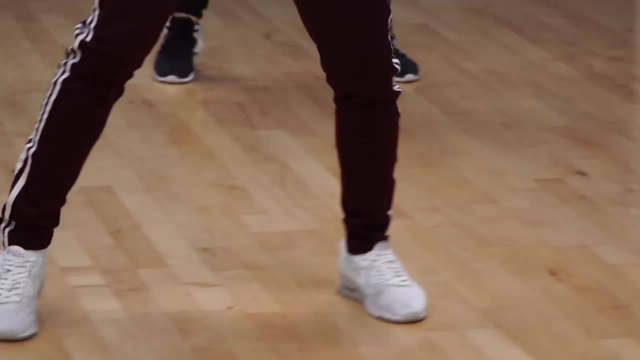 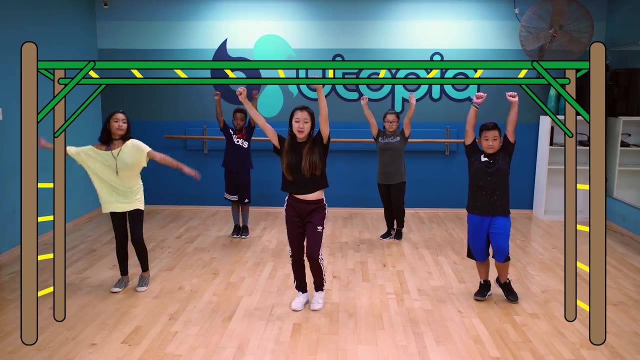 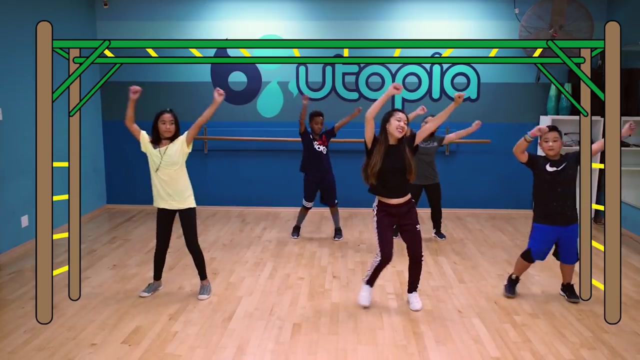 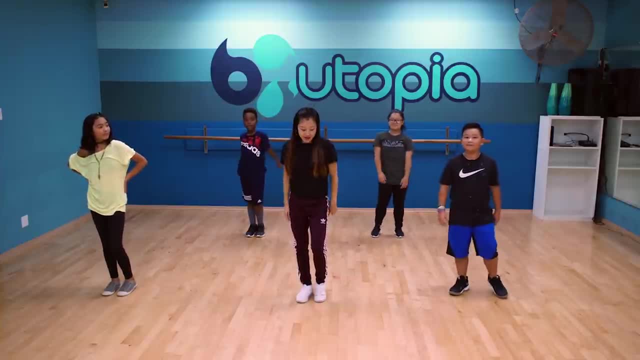 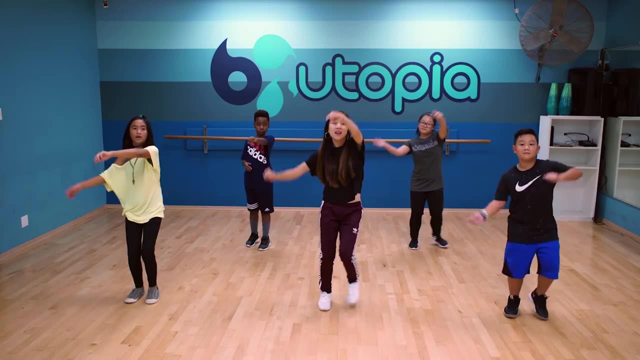 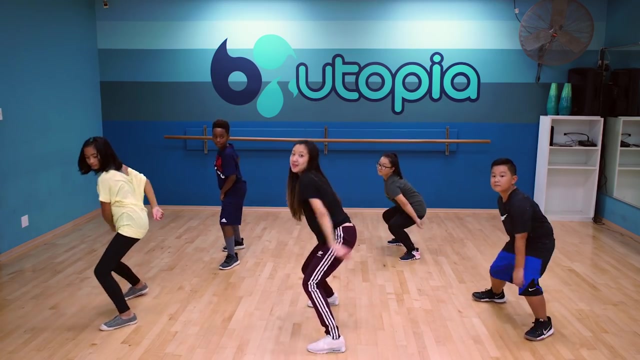 Nice, Can we try from jump in the catalog? Yeah, Here we go. Five, six, seven, Eight, jump in the catalog, Drive, drive, drive. then hang to this side, hang to that side. Nice, From here, take this foot. you're gonna step down together, down together, down together. 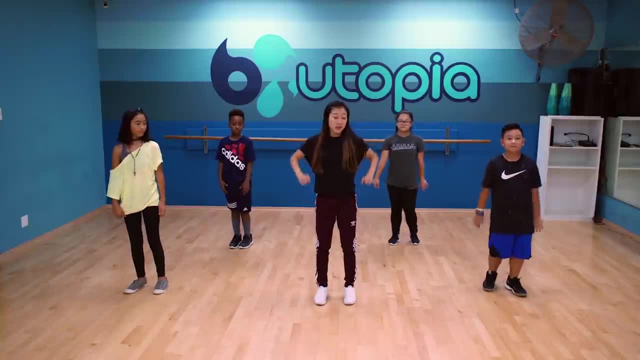 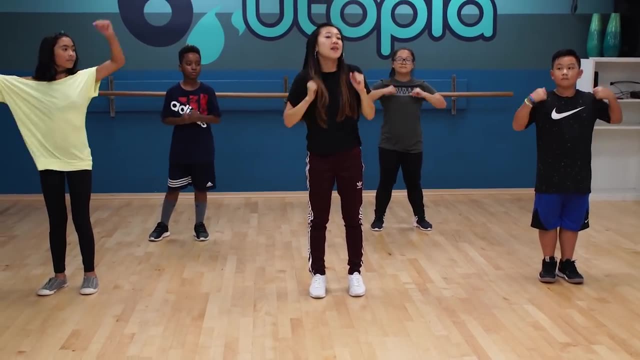 and down together. and then my arms, like we're pretending, like we're like scooping ice cream. So you're just gonna go down, down, down, point down, Hey leg, I'm gonna have some ice cream for you, whoop. 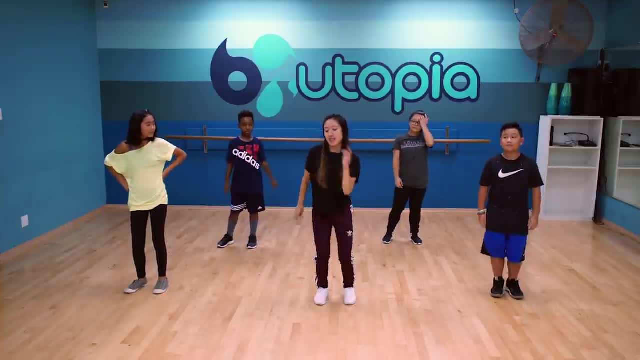 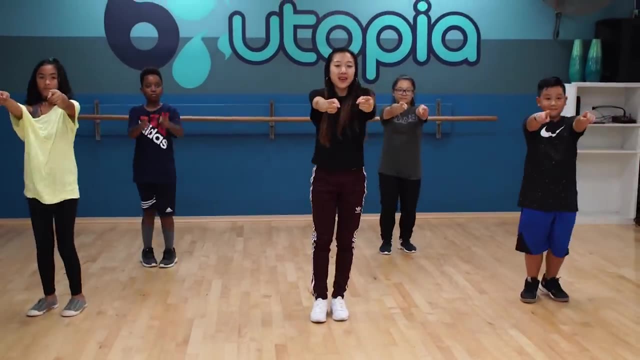 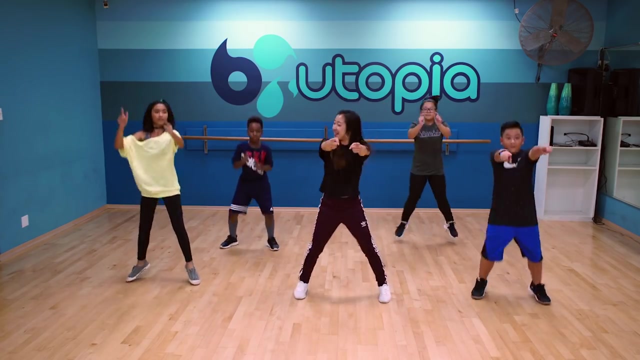 Down and point. cool, Can you try it with the feet? Let's turn to the side So you're gonna scoop down and point, down and point and after that we're turning on this leg. you're gonna go turn and then you're gonna dip, dip and jump. 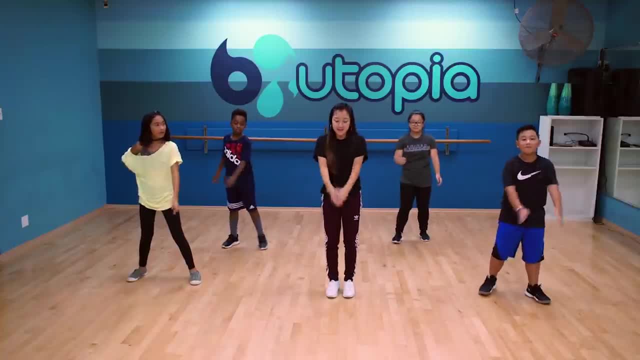 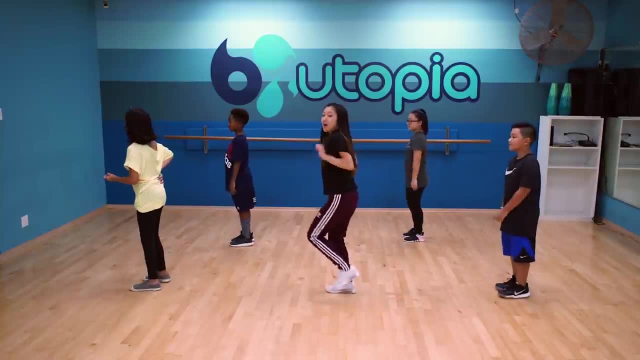 Yeah, Nice, Let's try that turn one more time. So we just, we just did. ah, let's see, We did the scoop, Scoop, Scoop, Scoop, Point, Scoop, Point, Turn Down. 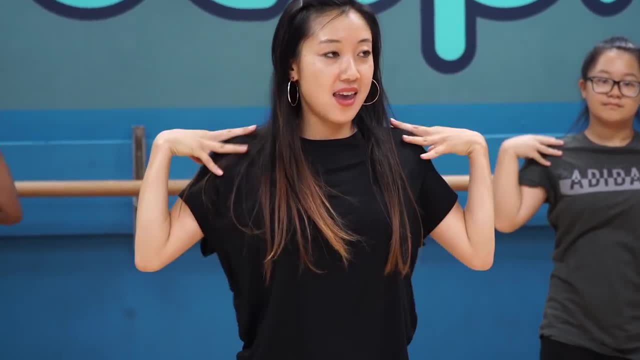 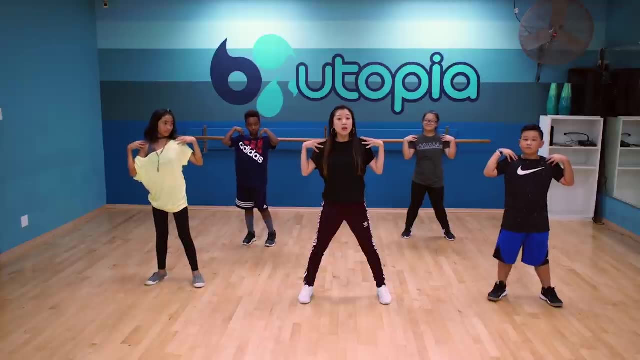 Point. And then you're gonna go cross. hey, hands on shoulders. We got some cool like shoulder pads with diamonds on it. Yeah, cause this song goes: cool jewelry and you're just gonna go shake, shake and 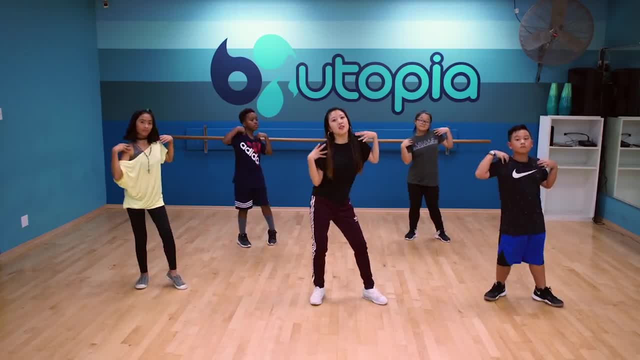 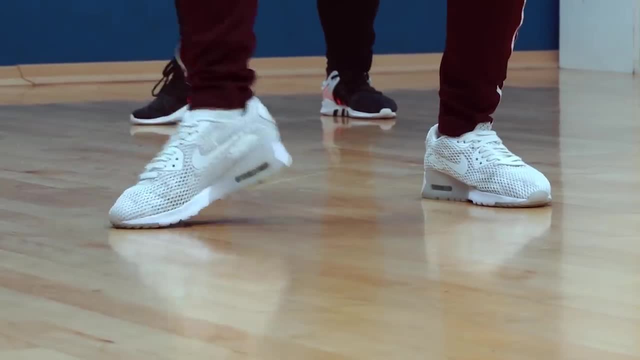 shake, shake, Yeah. shake your shoulders, shake your shoulders, Whoo Yeah. And then you see my heel. You're gonna show your heel like your nice. you know shoes, You got your Adidas, you got your Nikes. whatever shoes you have, they're dope. 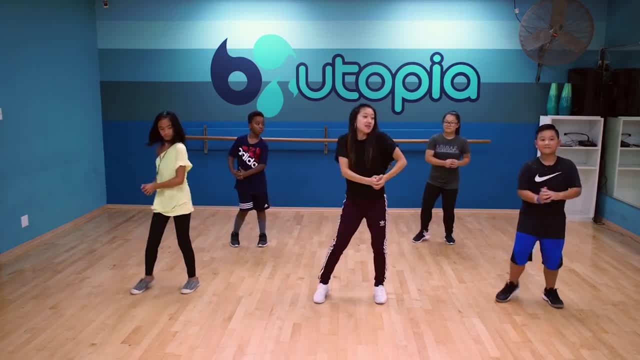 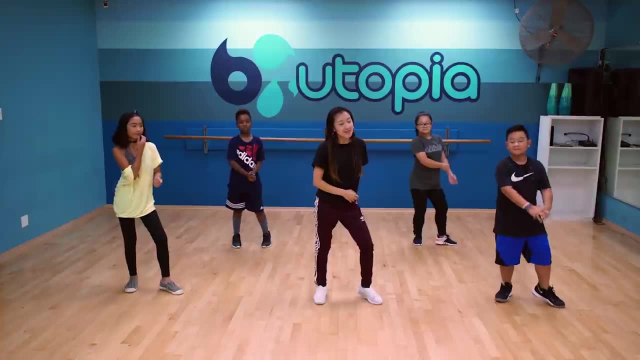 And then after that we're gonna make some ice cream. So you're gonna go swirl some ice cream, Yeah, Hey, Yeah Nice. And then after that we're gonna just go a little bounce, Bounce and then throw it. 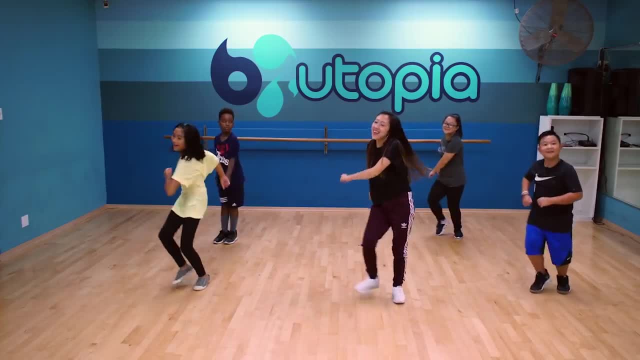 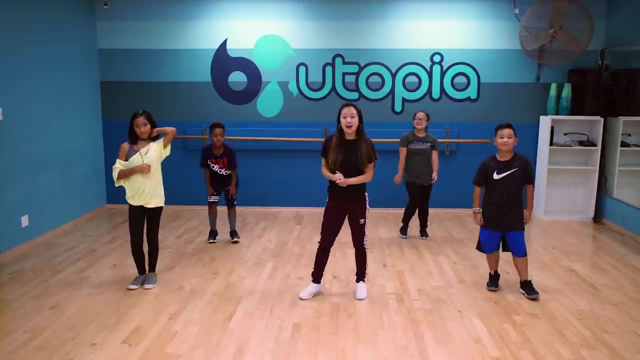 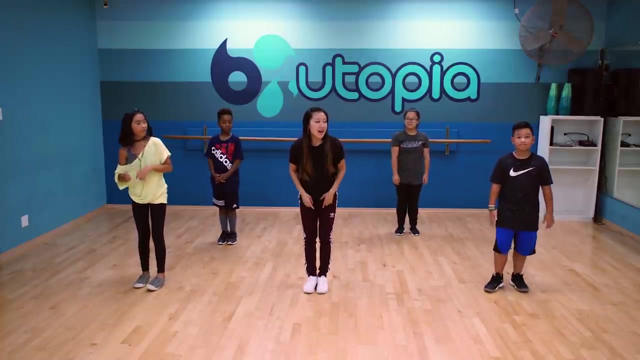 So go low and high, Low and high and low and high. Whoo, I think we could try from the top. Yeah, let's try from the top without music, and then we'll try it with music. Okay, 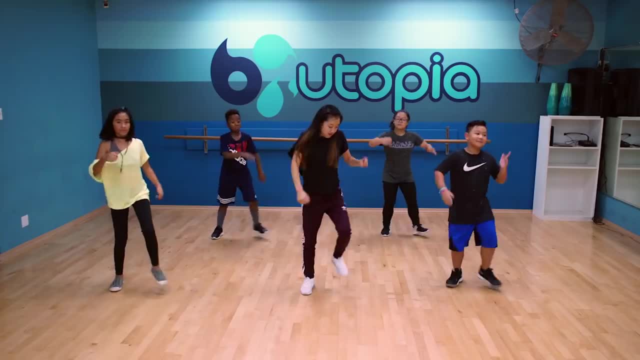 So we'll do it a little slower and then we'll do it with music. Here we go: Five, six, seven, eight, One, two, three and one, two, three. One, two, three and one, two, three. 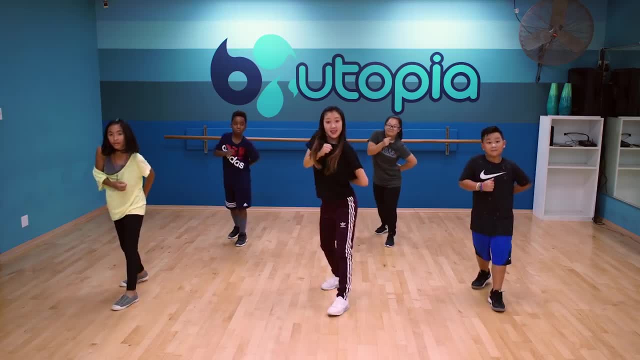 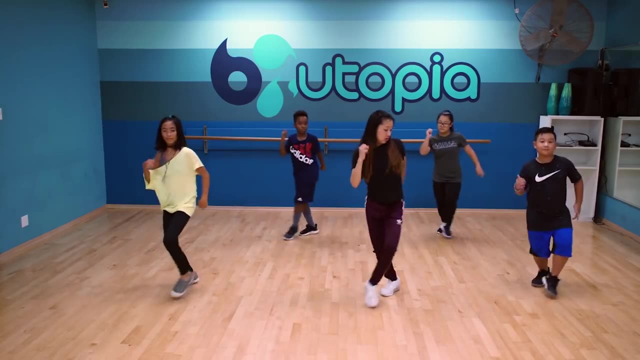 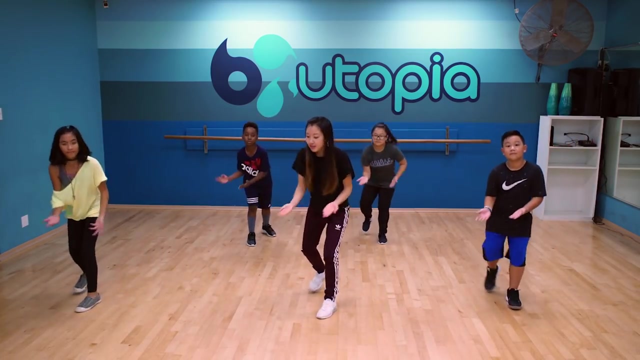 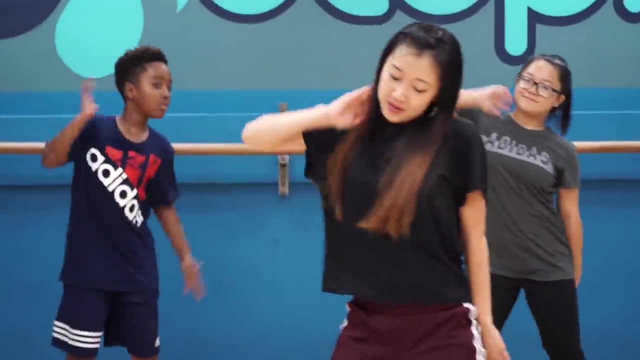 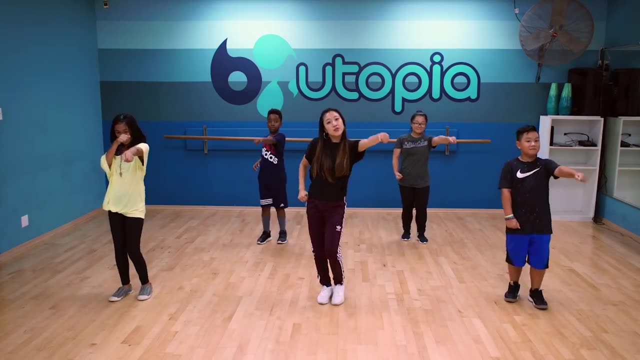 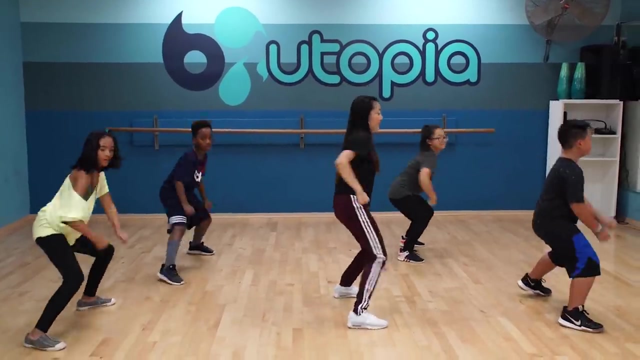 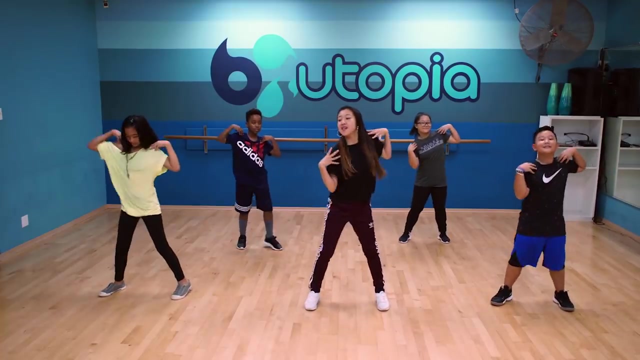 your pasta. Hey, And home, you're here. Now there's a new part. You're going to go jump in the Cadillac Drive, drive, drive, Hang, drive to the side, Hang to the side. Scoop and point. Scoop and point, Turn Down, point. Cool jewelry Shoulders and shoulders, And 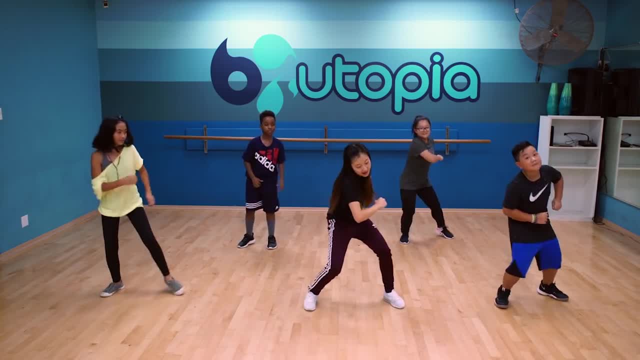 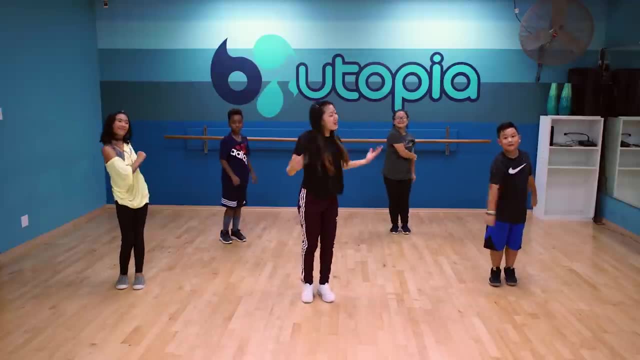 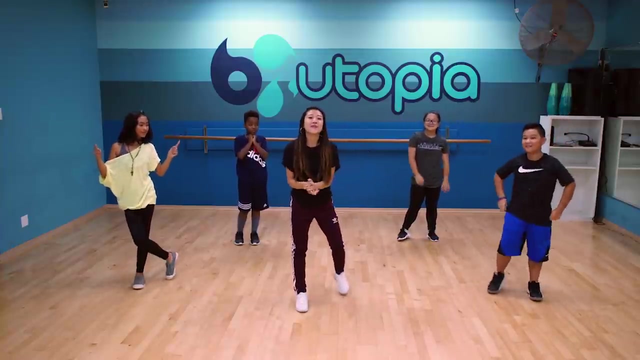 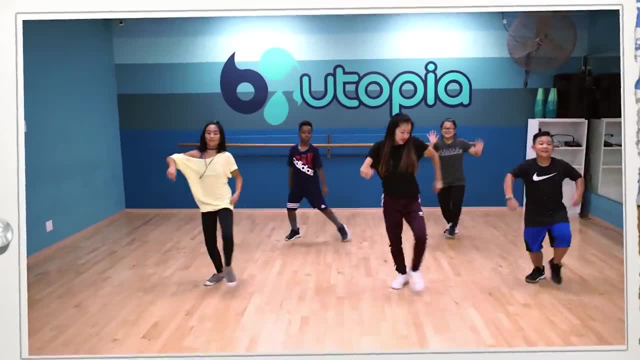 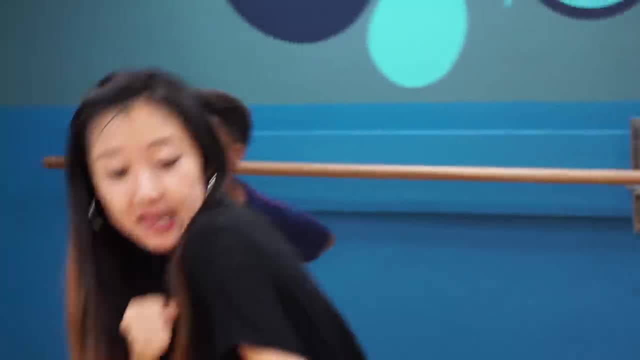 Hey, hey, hey, There is a condo in Manhattan, Hey there, hey, what's up? What's up? You and your friends invited. So go and get to dancing. Hey, sing it with a friend, Sing it, sing it for me. Come down and dance it with a friend. Dance it, dance it with me. 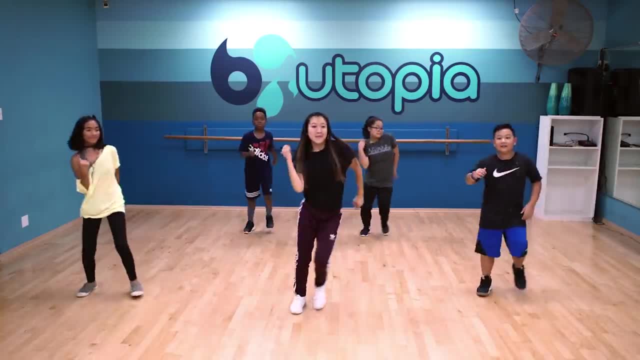 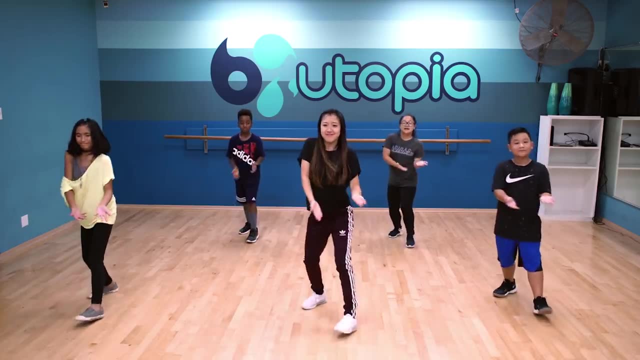 I have a bitch house in Miami Hang out in my jammies Lobster tail for dinner. Then we serve that scampi. You got it if you want it. Got it if you want it. Said: you got it if you want it. 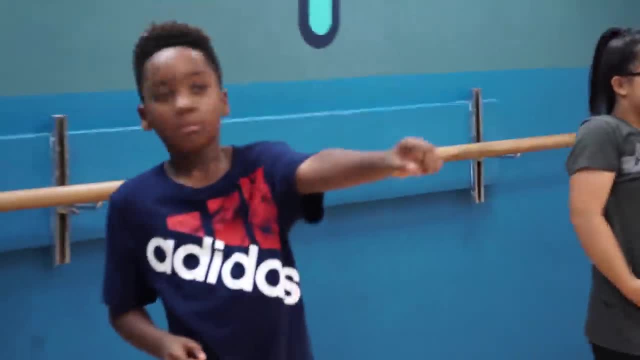 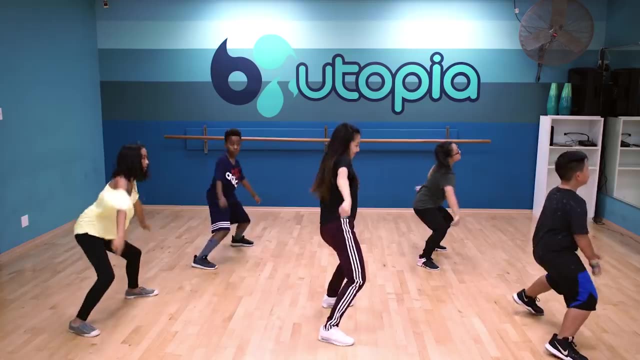 If you want it, then jump in a Cadillac. Hey, let's put some miles on it, Anything you want, Just to put a smile on it. You deserve it, baby. You deserve it all, And I'm gonna give it to you.